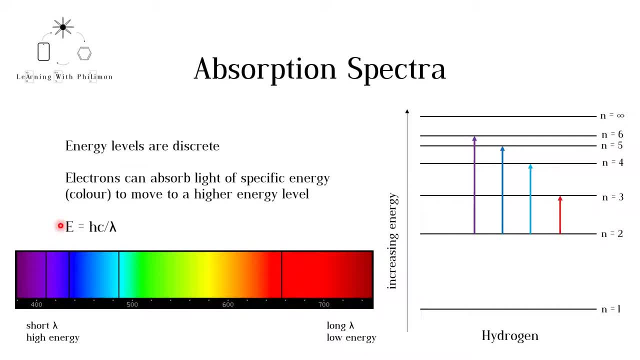 relationship between energy and wavelength. Energy E is equal to Planck's constant H multiplied by the speed of light C divided by the wavelength lambda. The larger the value of the wavelength, the larger the denominator, so the smaller the value of E. 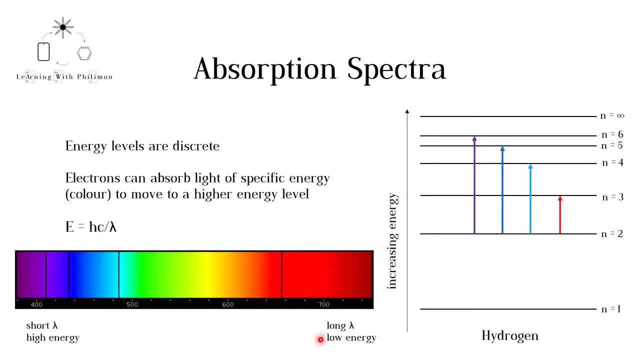 Red light has a long wavelength and therefore a low energy. Violet light has a short wavelength and therefore a high energy. This particular absorption spectrum belongs to the element hydrogen. If visible light is shone upon hydrogen atoms, the electrons will absorb specific wavelengths of light to transition to a higher energy level In the case of hydrogen. 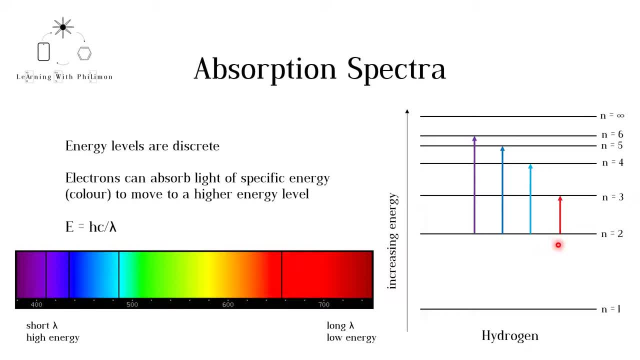 red light can be absorbed for the transition between energy levels 2 to 3.. Light blue is absorbed for the transition between energy levels 2 to 4.. Dark blue is absorbed for the transition between energy levels 2 to 5.. And finally, violet light is absorbed for the transition between energy. 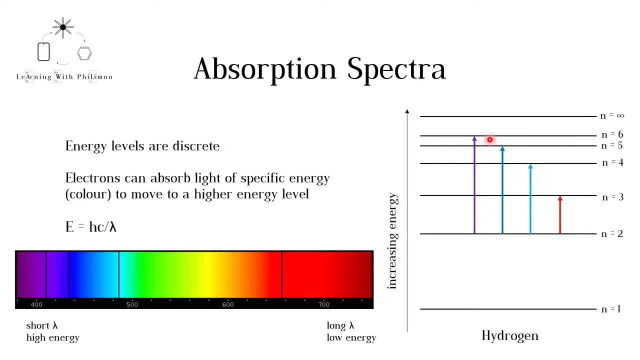 levels 2 to 6.. Note that there are black lines in the spectrum where these colors used to be. This is because only these four colors are absorbed. The rest of the colors would go through the sample of hydrogen and be detected Electrons. 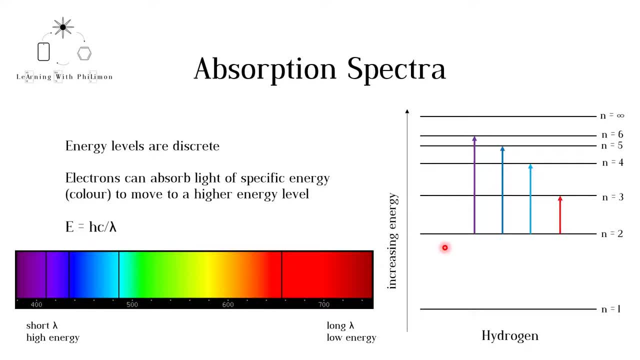 could transition from the first energy level to higher energy levels, but this energy is not in the visible part of the electromagnetic spectrum. Note that the gap between the energy levels decreases as the energy increases. This is described as the energy levels converging at higher energy. This is also evident in the absorption spectrum as the lines are closer. 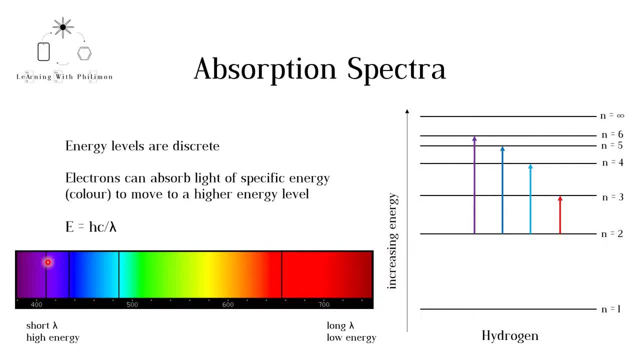 together as the energy increases. In the diagram only six energy levels are included, although there are more. The last line is labeled as infinite. If an electron absorbs energy to reach this point, it means it has left the atom. This is called ionization and will. 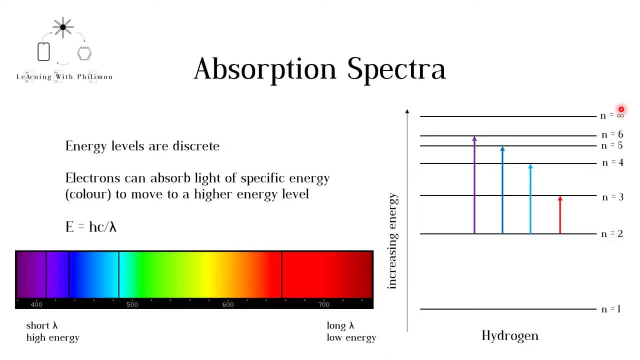 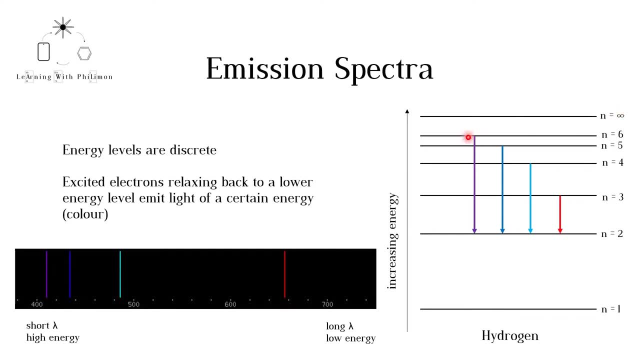 be discussed in the bonding and periodicity playlists. Emission spectra are very similar to absorption spectra. Electrons that have gained energy and transitioned to a higher energy level are called excited electrons. These electrons relax and transition back into a lower energy level. In doing so, they